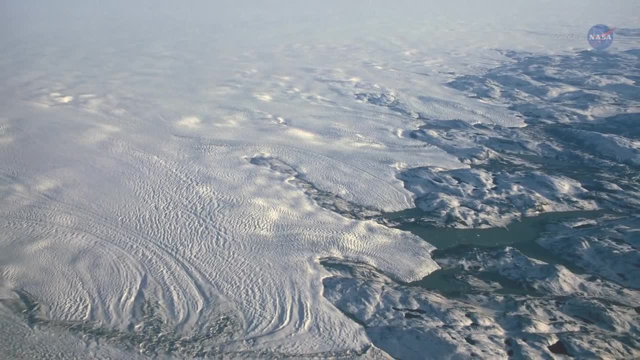 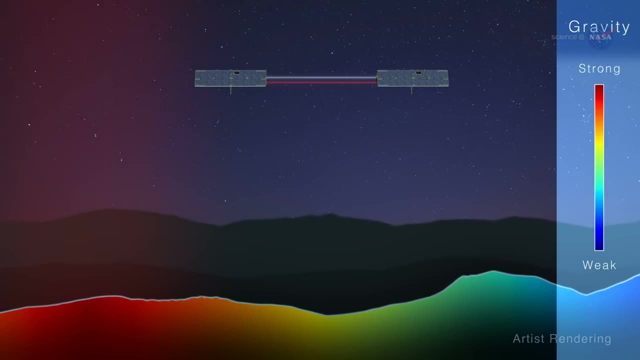 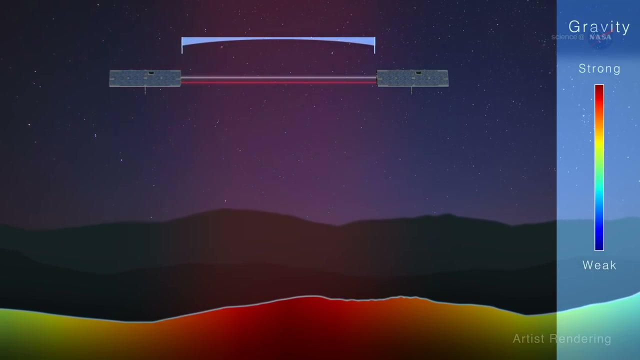 changing the forces controlling the orbits of the satellites. The two GRACE-FO satellites orbit about 135 miles or 220 kilometers from one another, with one satellite leading the other. If the lead satellite encounters a change in gravity, its speed changes, as does its relative distance to the trailing satellite. 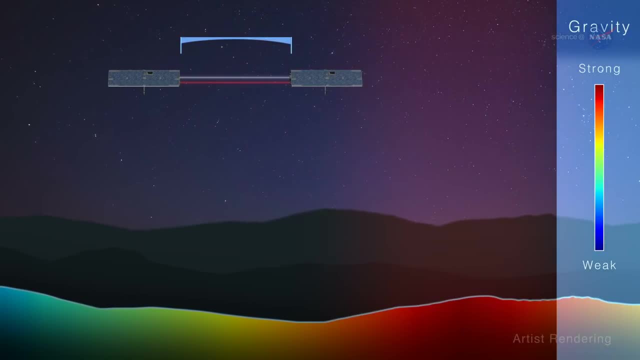 Microwaves and lasers are used to measure the tiny changes in distance between the two satellites. GRACE-FO satellites are used to measure the tiny changes in distance between the two satellites. GRACE-FO satellites are used to measure the tiny changes in distance between the two satellites. 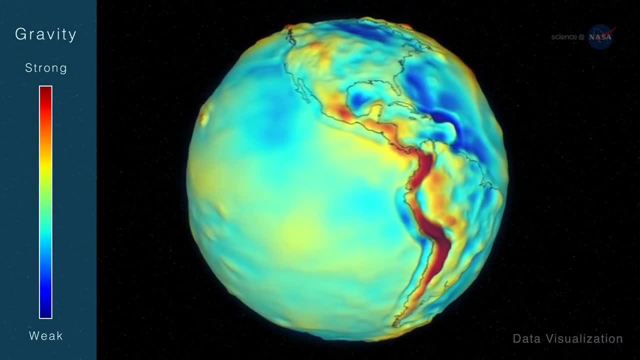 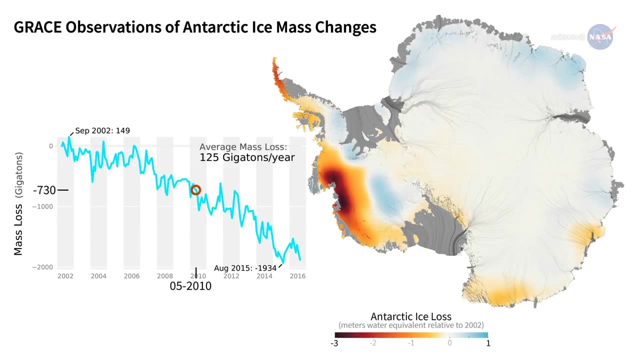 By taking measurements of multiple passes over the same location, scientists can create maps of that location's gravitational field Over Earth's frozen regions. this information shows where ice sheets and glaciers are gaining or losing mass Over Earth's frozen regions. this information shows where ice sheets and glaciers are gaining or losing mass. 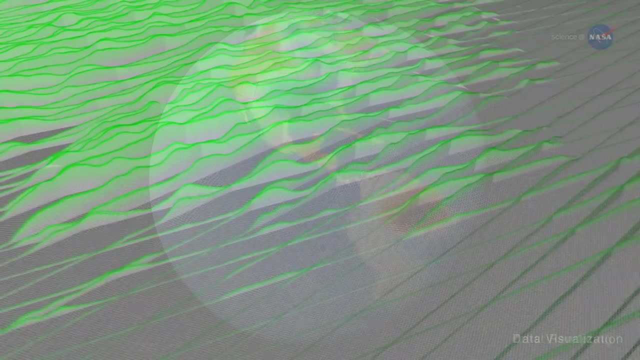 While GRACE-FO gives a global view of changes in the distribution of mass on Earth, ICESat-2 will provide complementary measurements of ice sheet height. ICESat-2,, which is scheduled to launch in the fall of 2021, will provide complementary measurements of ice sheet height. 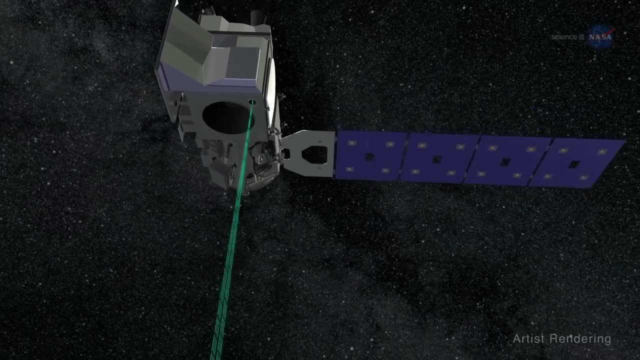 ICESat-2,, which is scheduled to launch in the fall of 2021, will provide complementary measurements of ice sheet height. The ICESat-2 satellite, which was integrated into NASA's Goddard Space Flight Center in the fall of 2018,. 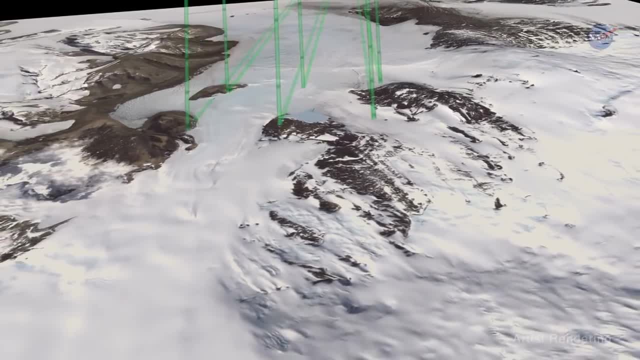 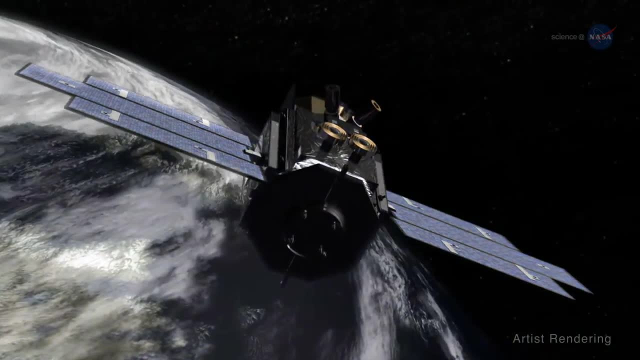 is a single satellite operated out of NASA's Goddard Space Flight Center that uses its laser to shoot beams of light to earth. Scientists can determine a location's elevation by measuring the travel time of these laser pulses- The original ICESat mission, which operated from 2003 to 2010,. 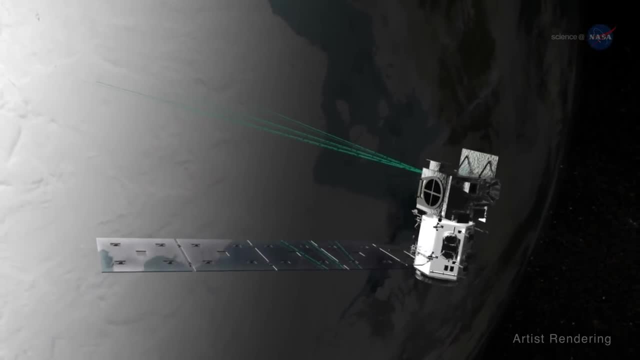 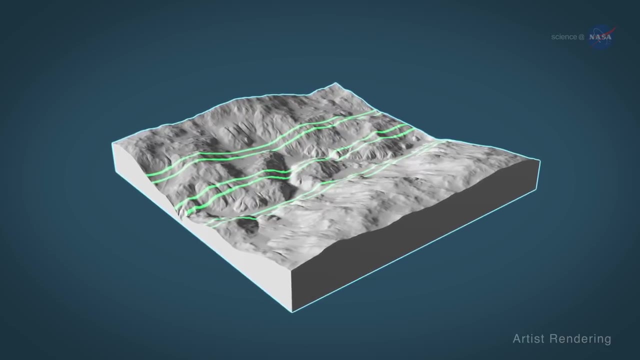 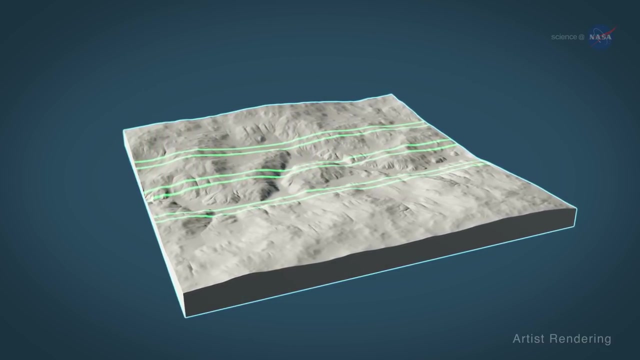 used a single laser beam. ICESat-2 uses six beams to improve accuracy and resolution. Using six beams gives scientists multiple points of data within the laser's footprint, allowing them to measure the slope of an area and then separate static slope data from the area's changes in elevation over time. 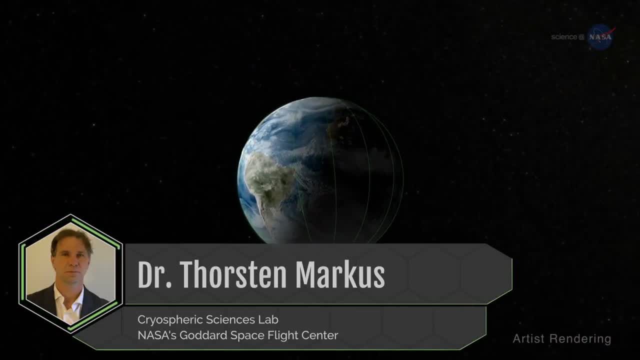 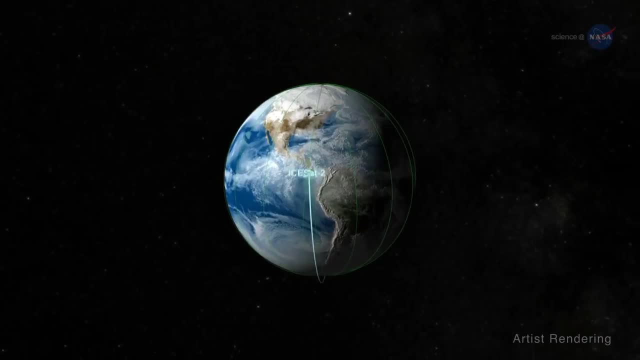 Why is this elevation information important? Dr Torsten Markus, chief of the Cryospheric Sciences Lab at Goddard, explains: ISAT-2's orbit repeats measurements every 90 days, which allows us to see change while also helping to determine the drivers of that change. 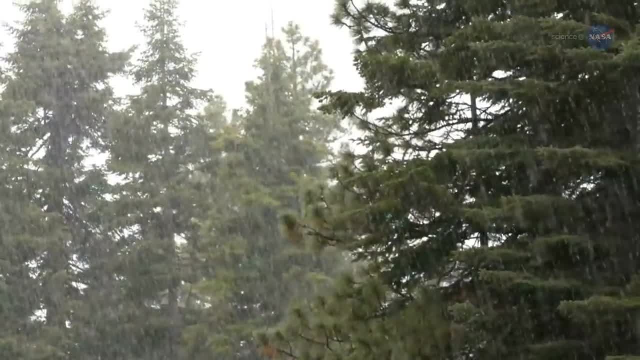 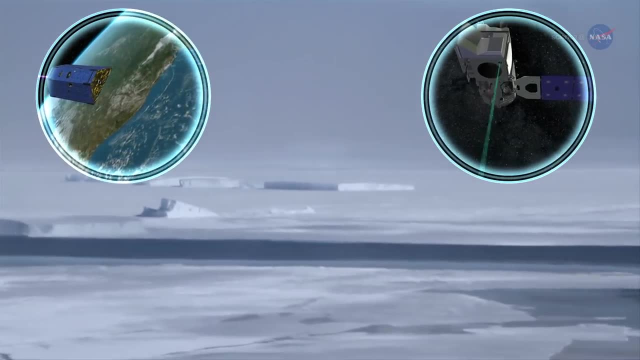 For example, is melting in one region, balanced by snowfall in another. GRACE-FO and ISAT-2 will be the newest NASA missions being used to study the cryosphere and its role in the Earth system, In addition to their cryospheric objectives.